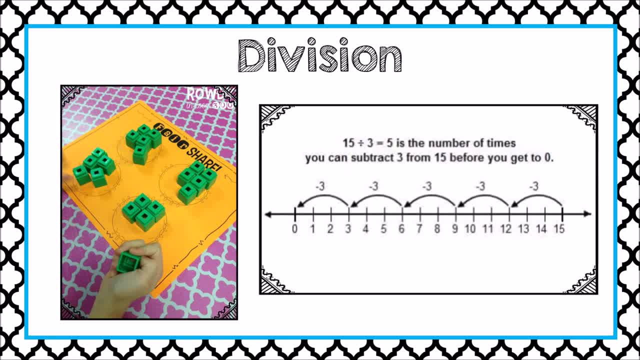 equal groups. Or, secondly, we could be doing repeated subtraction or repeatedly taking away groups. As I model the area, model division strategy, I am going to think about the second type of division, where I repeatedly take away groups until I am left with nothing. 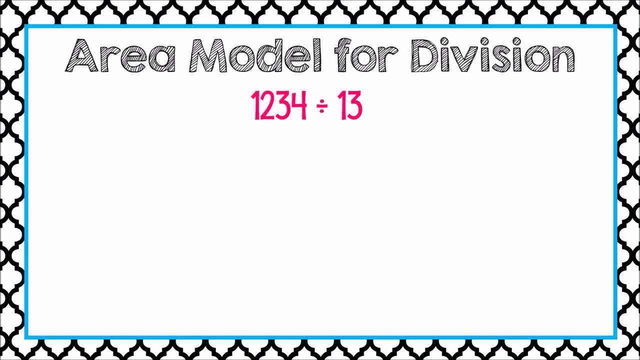 When I use the area model for division, I start with a quick brain dump. This is where I write down everything that is in my brain. My brain dump will be about the number that I am dividing by, in this case, the number 13.. Although this brain dump is for a division, 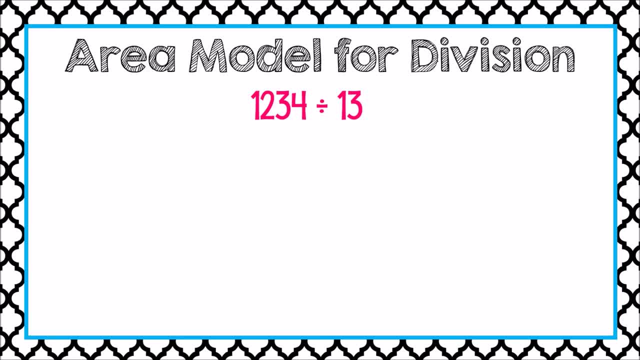 problem. I am going to think about multiplication for a minute. Soon you will see why this is helpful. So, for example, I know 13 times 1 is 13,, 13 times 2 is 26, and 13 times 3 is 39. What else do I know about 13?? Well, if I know. 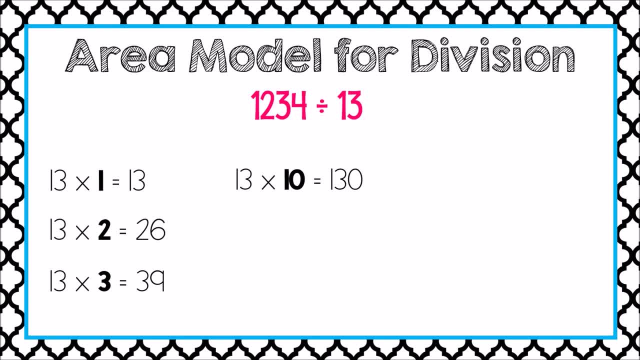 13 times 1, it helps me know 13 times 10,, that's 130.. If I know 13 times 2,, it helps me know: 13 times 20,, that's 260.. And if I know 13 times 3,, it helps me know 13 times. 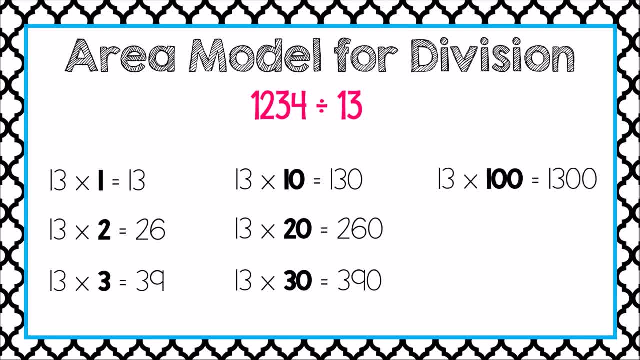 30,, that's 390.. Hmm, well, I also know 13 times 100 is 1,300, but I really don't need to know that for solving this problem. Now that I've thought about ways to multiply 13,, I'm going to use that to help me divide. 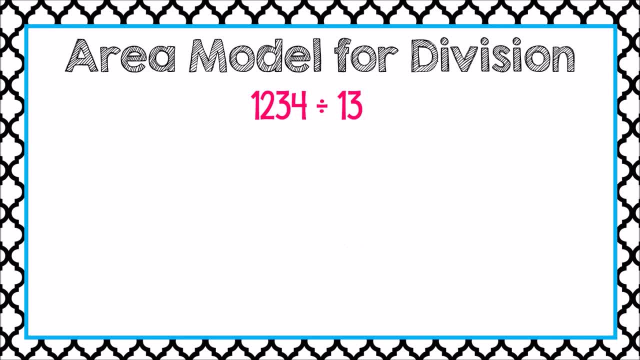 by 13.. Remember, multiplication and division are related. I start by creating a rectangular area model. I make a space for each place in the number that I am dividing, which is 1,234.. I write this number in expanded form: 1,234.. 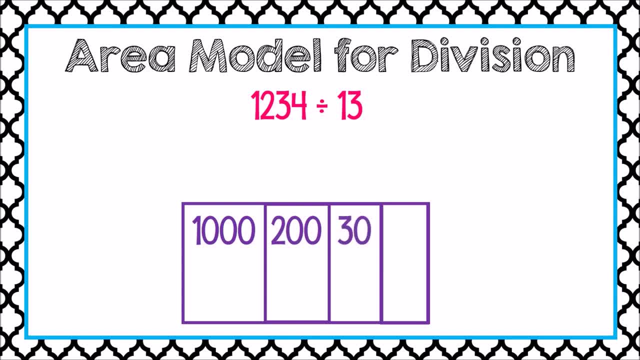 Gesch krypt. I divide this by 13.. Now that we've broken up our number by its place value, let's divide. I know 13 can be repeatedly taken from 1 thousand or divided into 1 thousand, at least once. 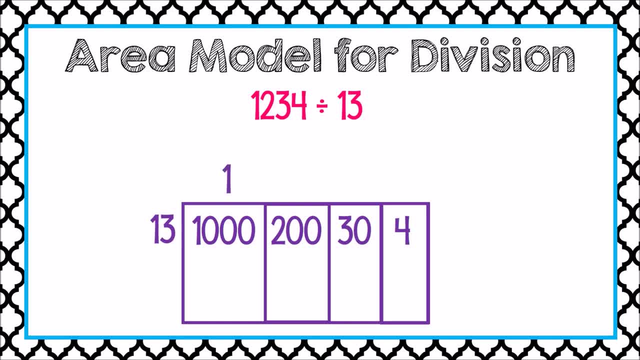 time, because 1 times 13 is thirteen. Wow, that's not nearly enough. I know that 13 can be repeatedly subtracted from 1 thousand at least ten times. Well, myнитansencom, I know that 13 can be repeatedly subtracted from 1 thousand at least ten times because. 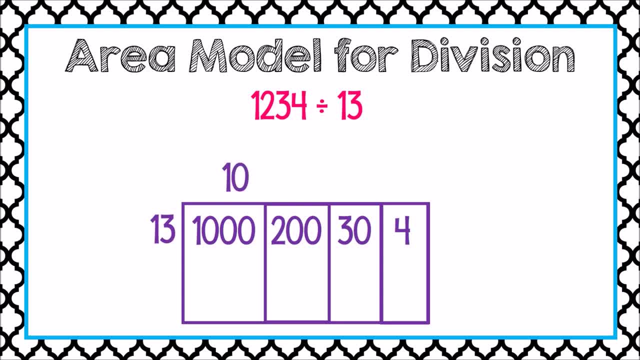 1 times 13 is 13.. I know that 13 can be repeatedly subtracted from 1 thousand, at least 10 times. Well, myнитansencom, Well, myнитansencom, because 10 times 13 is 130. Okay, well, 13 can divide into 10, into 1020 times, because 13 times. 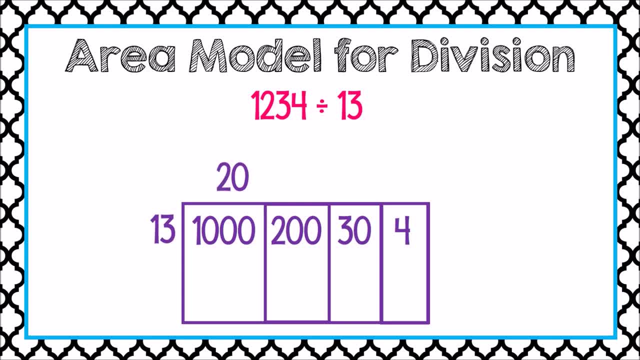 20 is 260.. Ugh, these numbers just aren't big enough. Let me try a bigger number. Hmm, how about 70?? Let's see if I can divide 13 into 1000, 70 times. In other words, can I repeatedly subtract? 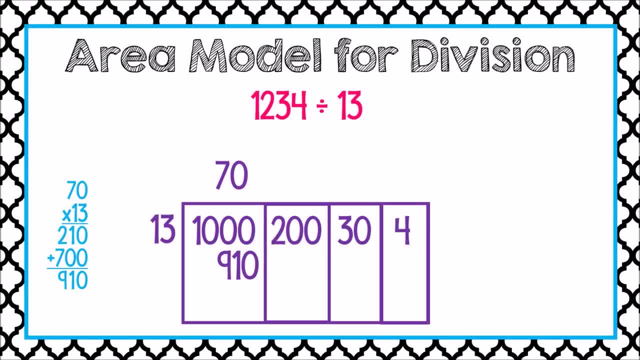 13 from 1000. 70 times, 70 times 13 is 910.. When I take 13 away, 70 times, that's 910.. Well, now I'm left with 90. Let's move that over into the next place. Now, how many times can I divide 13 into? 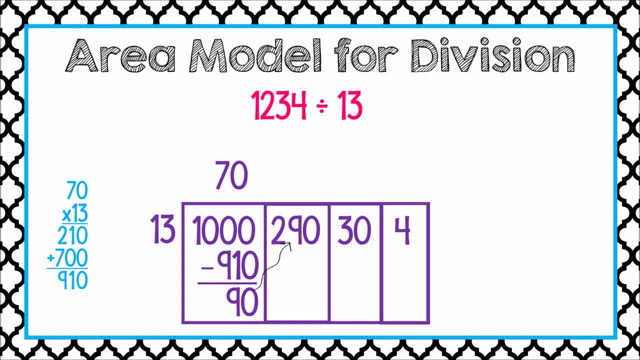 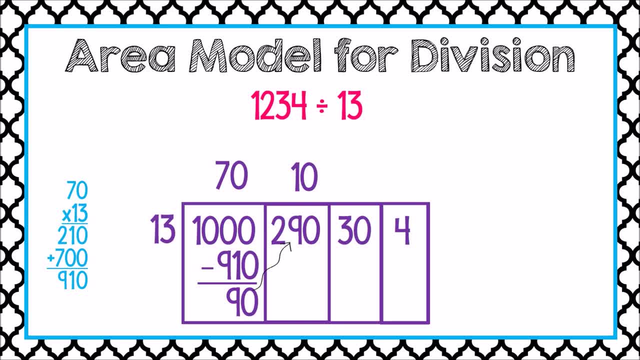 do that. I can't do that. Okay, 13 times 10 is 130.. I could still take away more. I could try taking 13 away 20 times 20 times 13 is 260.. Let's do that. I have 30 left. I'm going to move 30 over. 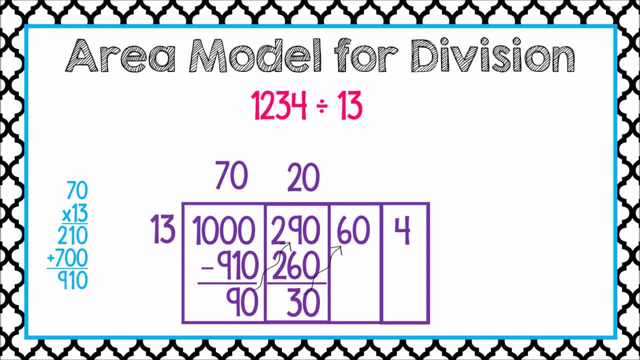 to the next place, making this 30 a 60. Hmm, 13 can definitely divide into 60 two times, because 2 times 13 is 26.. Let's see if 13 can divide into 60 three times. Yep, 13 times 3 is 39.. Now I have 21 left. Let's move that 21 to the last. 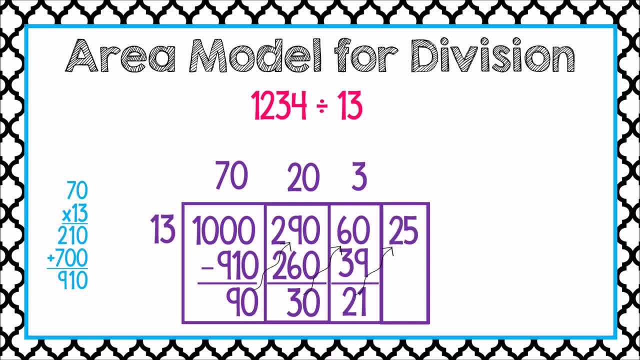 place, making this 4 a 25.. I can divide 13 into 25 one time. 13 times 1 is 13. And we have a remainder of 12.. Wow, look at all the times I was able to divide 13 into the next place. 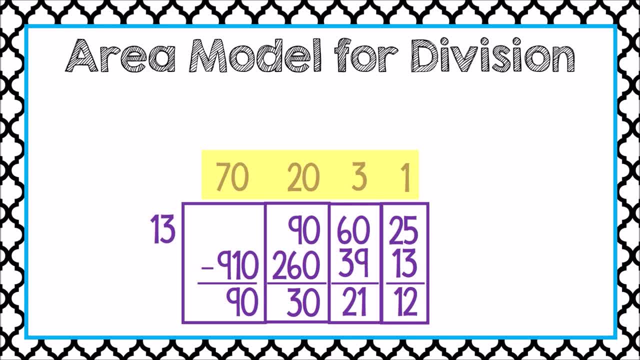 Now, if I look at the number 1234, that means I repeatedly subtracted 13 from 1234 this many times. When I add all of these numbers together, I find out that 13 divides into 1234 94 times with a.